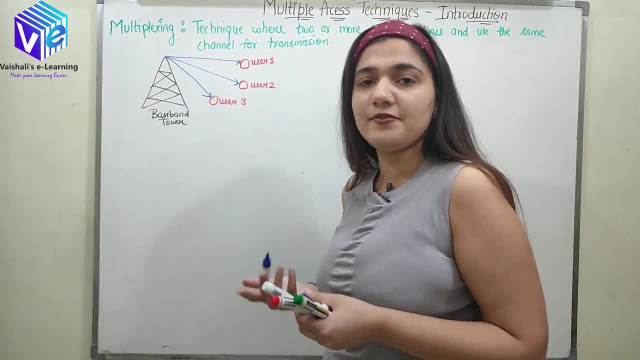 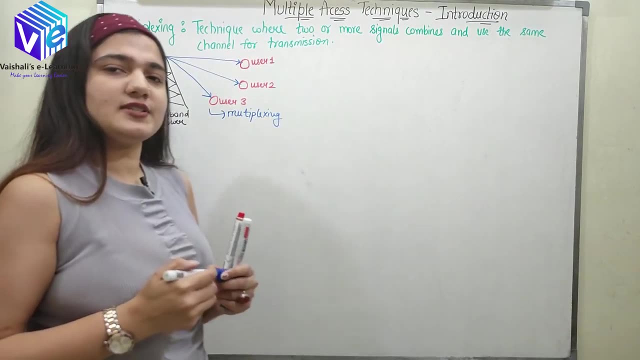 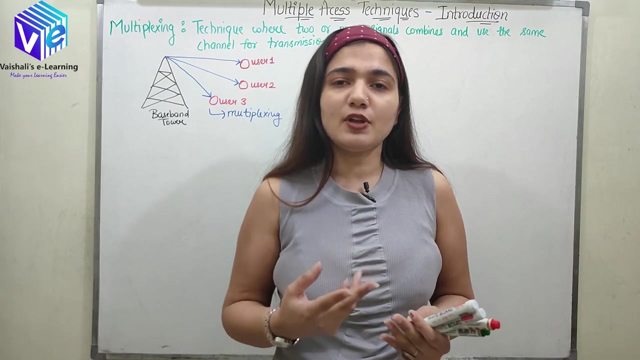 the same medium. So the medium or the channel is the same, which is the air. So now this is called the multiplexing. All of you must have seen this in your real life as well, if two of you are talking simultaneously with two different people. So now, that time, what would happen? It is going through the 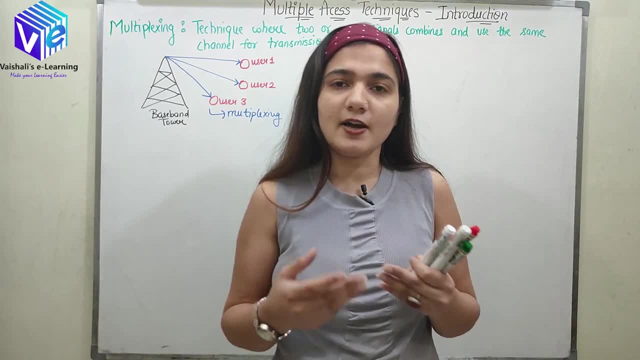 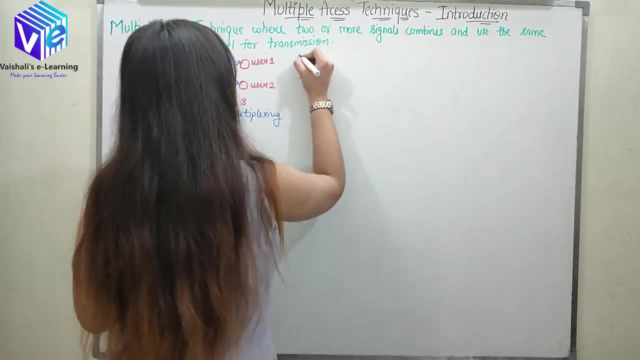 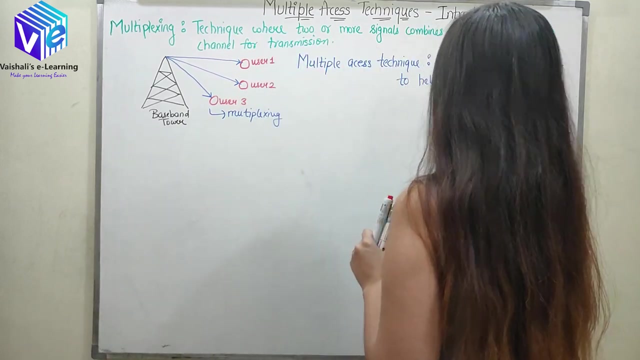 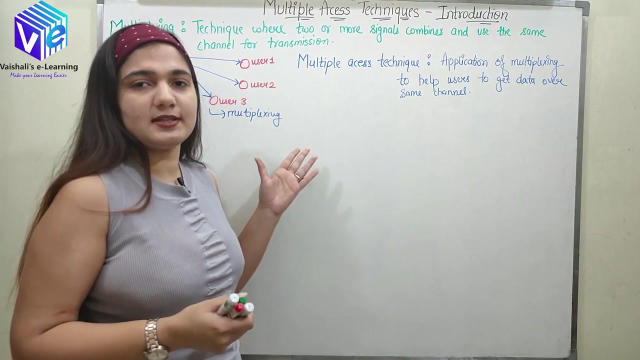 multiplexing, Your signal and your friend's signal are combined and going through the same channel, which is the air. So now, if I talk about the multiple access technique, So now multiple access technique is the application of multiplexing. So whenever I apply this multiple 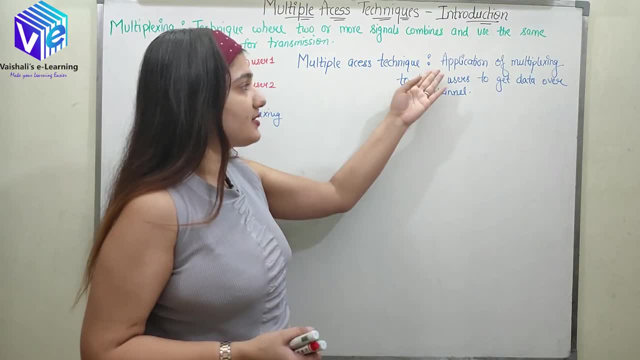 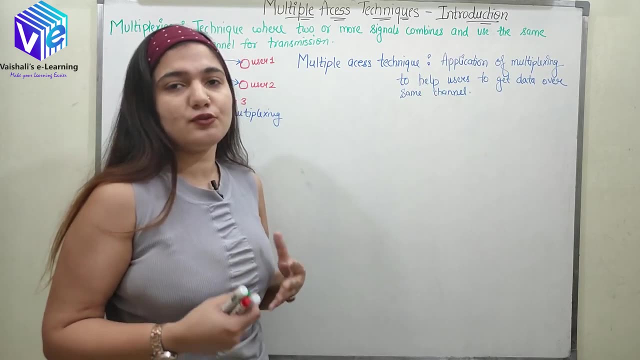 multiplexing technique. it is called multiple access technique and it is the application of multiplexing to help user to get data over the same channel. So lets take an example of Wi-Fi. so all of you must have used Wi-Fi in your life. If you are using Wi-Fi with, 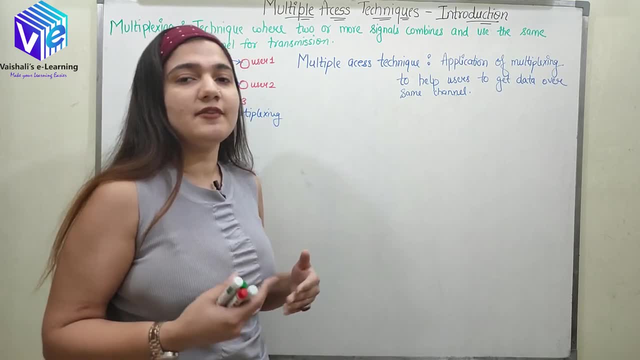 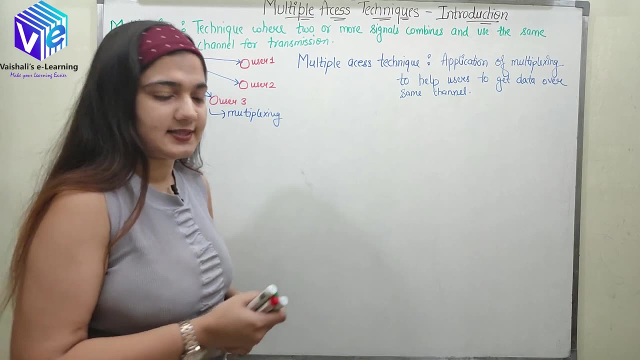 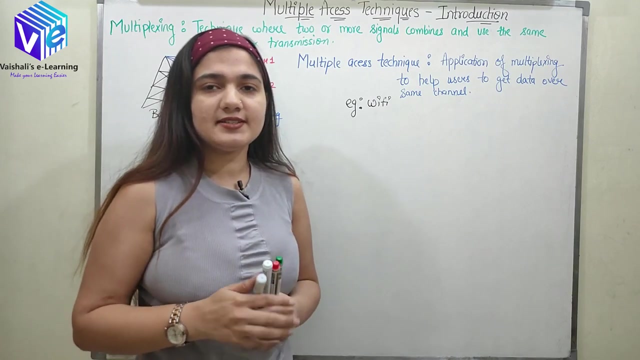 four other people combined. So what would happen? Leaks. It is like a series of three that Wi-Fi is sharing the same channel, which is the air. so same channel is shared with the help of multiple access techniques. so I can say the example would be Wi-Fi, so it's the most simplest example. after that we will discuss about. 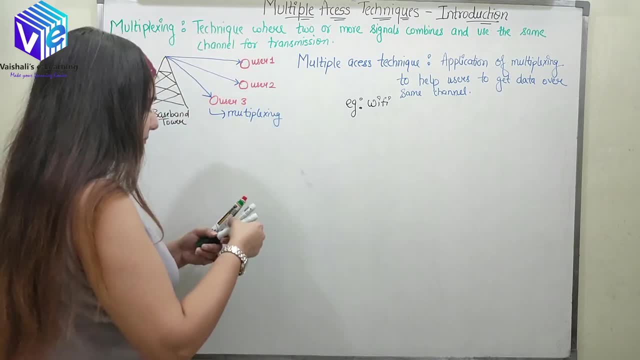 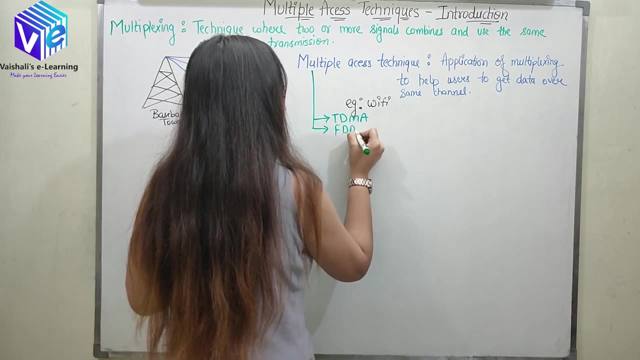 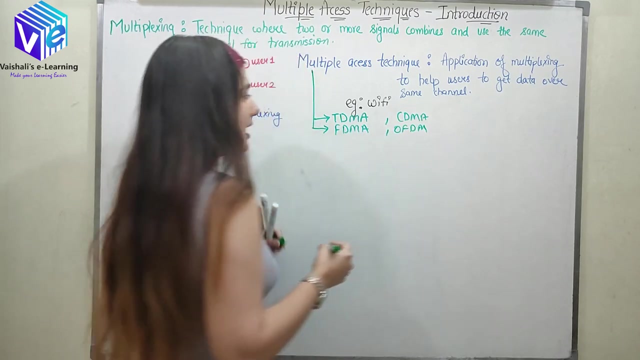 the types of multiple access techniques, so the type that it has various types. so it has the first type, which is called TDMA, FDMA, CDMA, OFDM and some other types are also there, so I'll discuss about them also. so first come to FDMA. 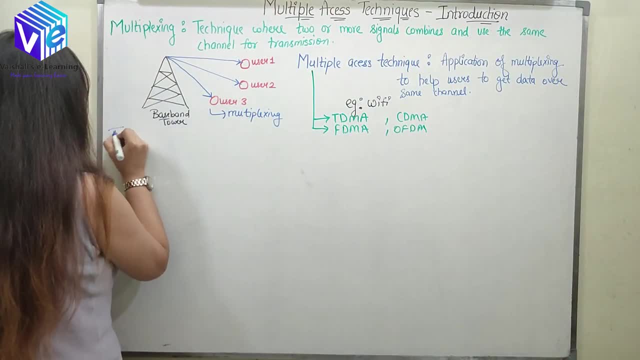 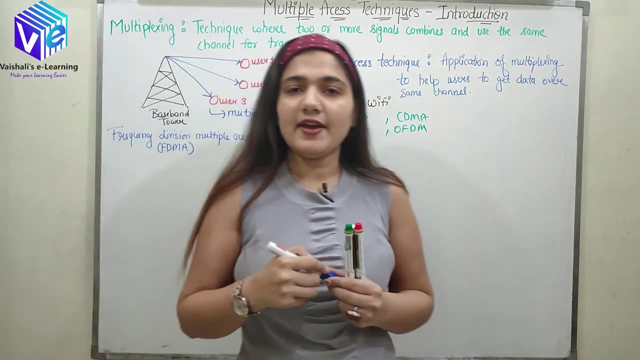 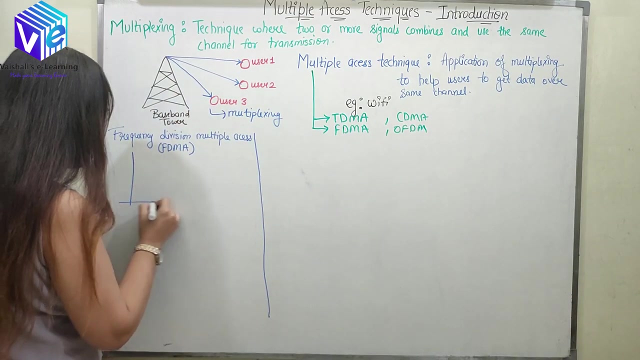 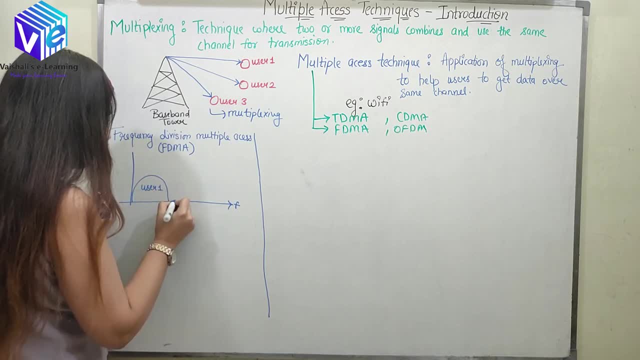 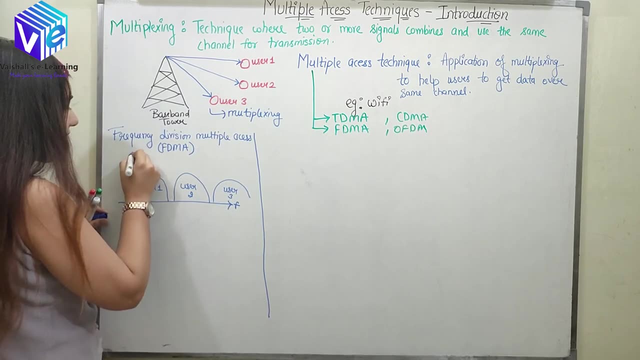 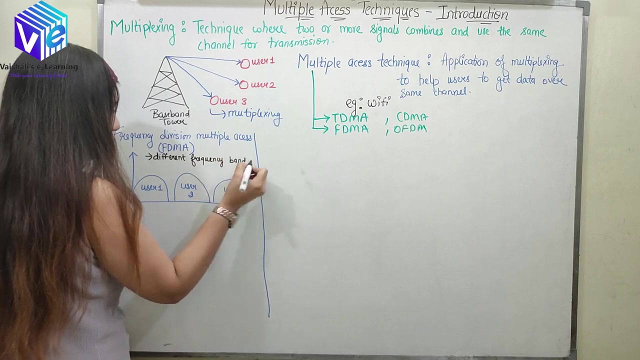 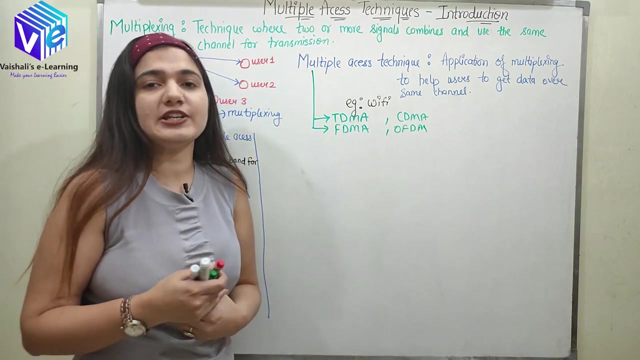 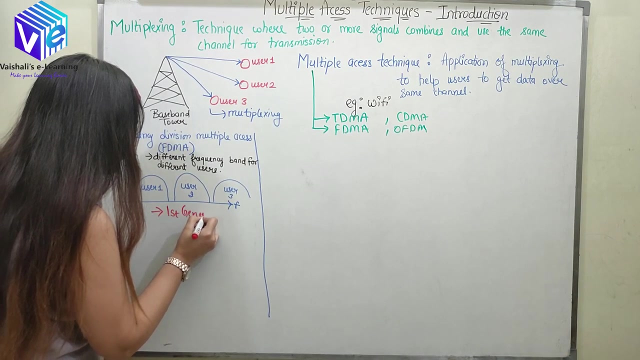 now, if this is my user one, then this would be my user two and similarly, this would be my user three. so I have different frequency bands for different users. so now this was the first generation. I hope you all have heard about 1G, 2G, 3G and 4G, so this is called the first generation, or 1G, so in 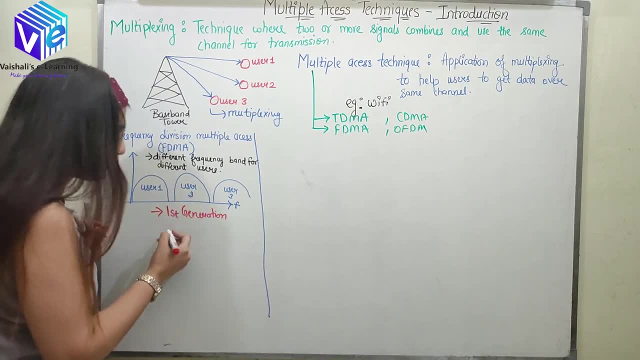 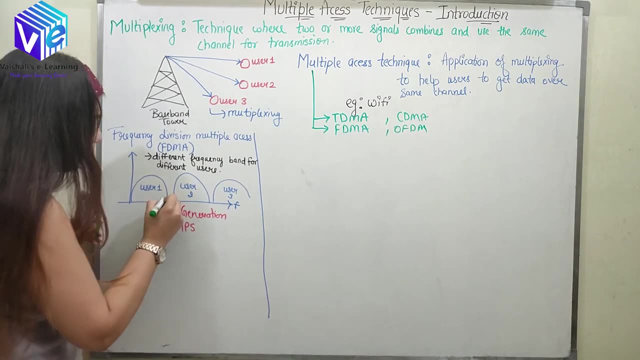 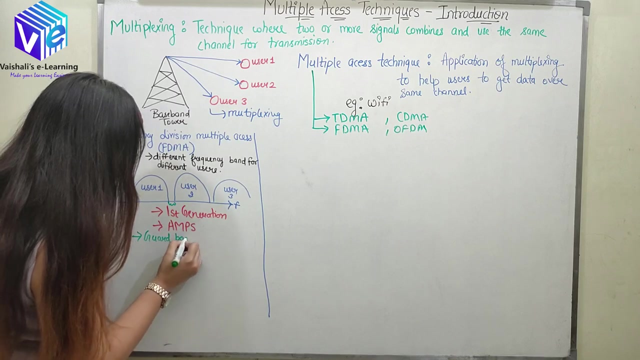 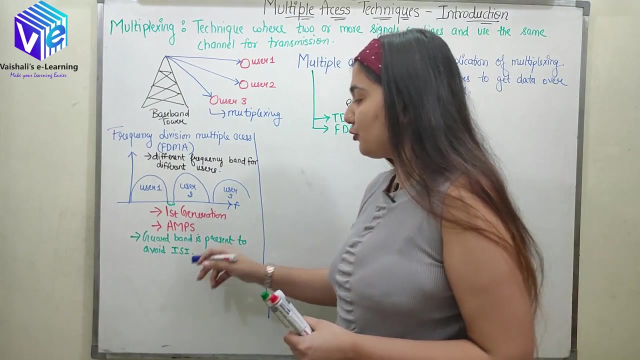 first generation data transfer, FDMA, was used, so which was AMPS. so now I hope you can see I have made a gap between user 1 and user 2, so this is called the guard band. so now by guard, guard band is present. guard band is present to avoid ISI and 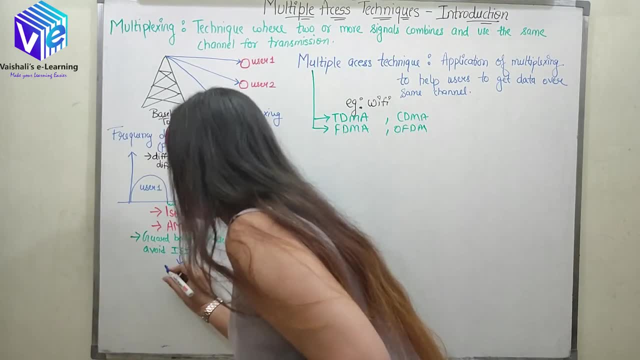 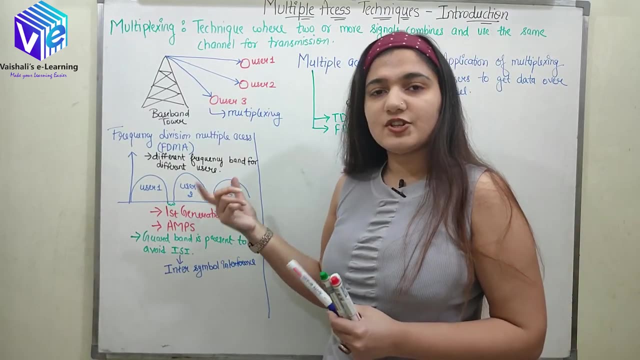 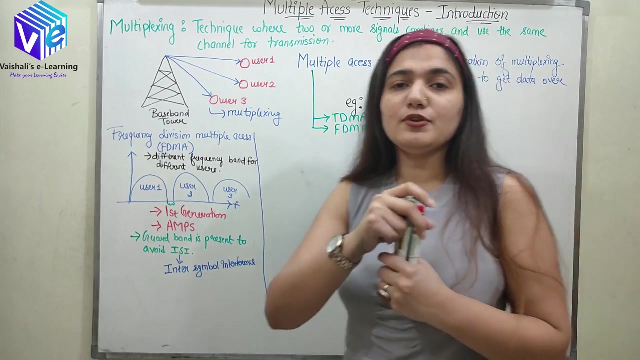 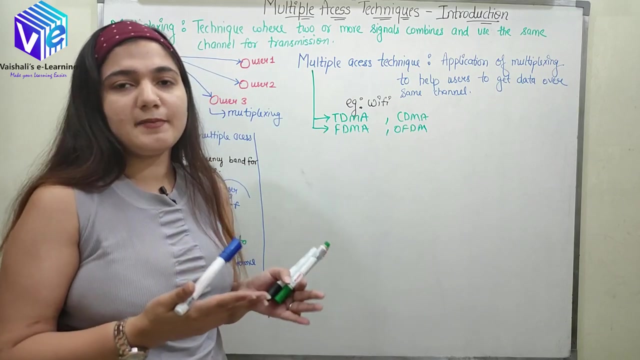 what is ISI? I hope you are aware of this term. this is called inter symbol interference. so now in this frequency division- multiple access- I have different frequency bands for different users. I hope you know that frequency bands are really costly and if I am a particular frequency band for a particular user, this process becomes really costly. 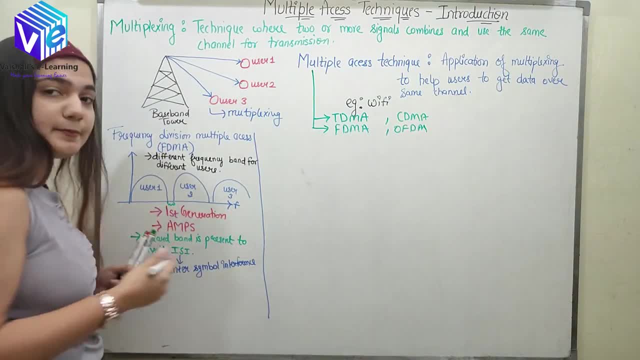 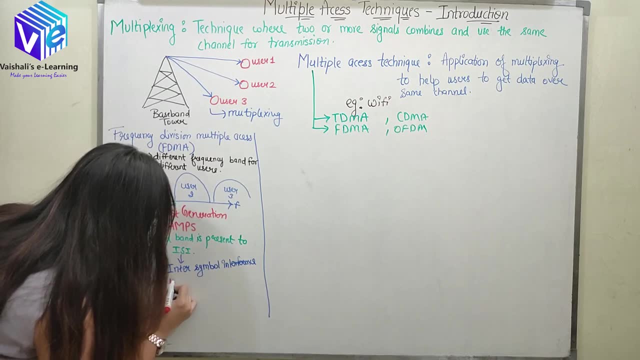 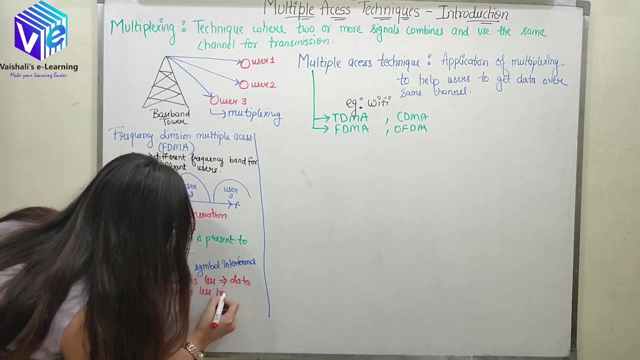 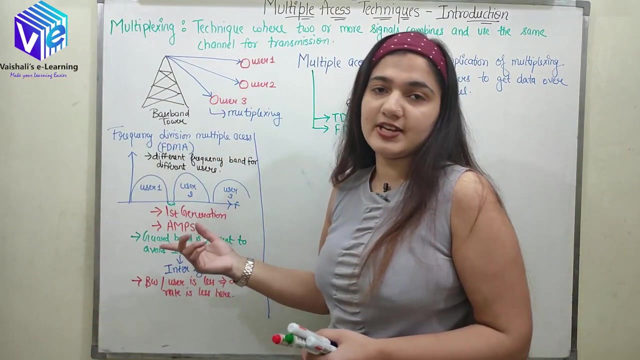 So the frequency band would be less. If the frequency band per user is very less, then the data rate would be less. So if the bandwidth per user is less, which implies data rate is less here, So plus the addition of guard band is destroying my bandwidth efficiency. 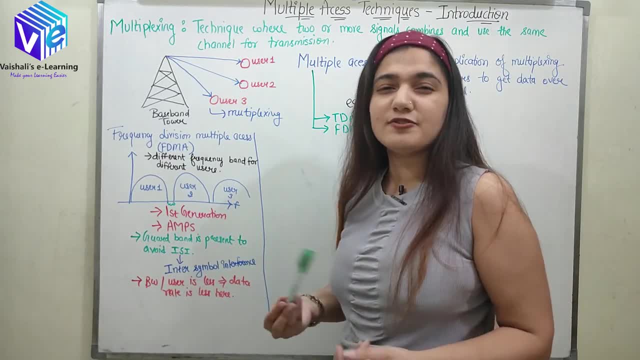 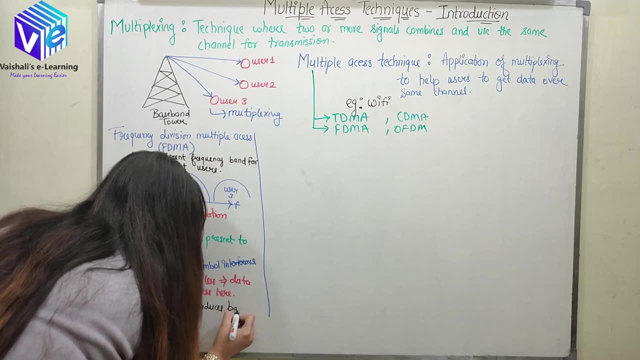 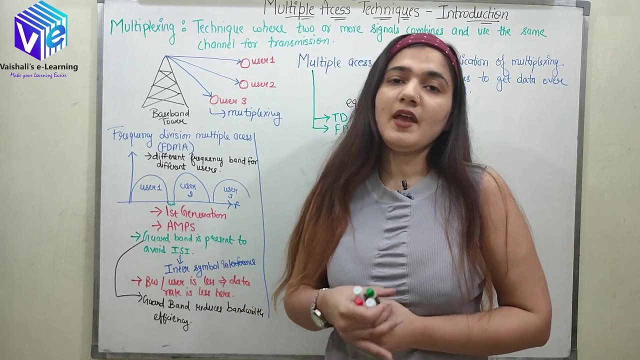 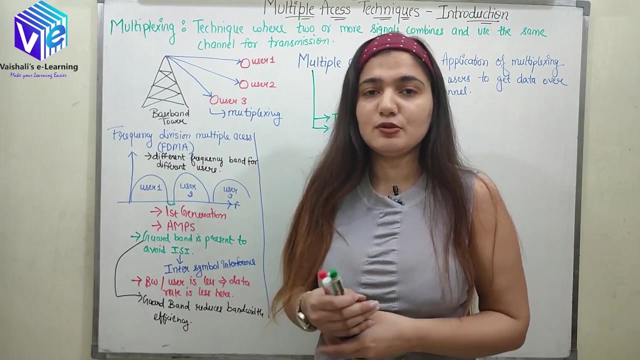 The presence of guard band is not suitable for my bandwidth to be very efficient. So now, guard band reduces bandwidth efficiency. As I already said a lot of time, the bandwidth spectrum is costlier, So when the companies are using bandwidth, They have to purchase it. 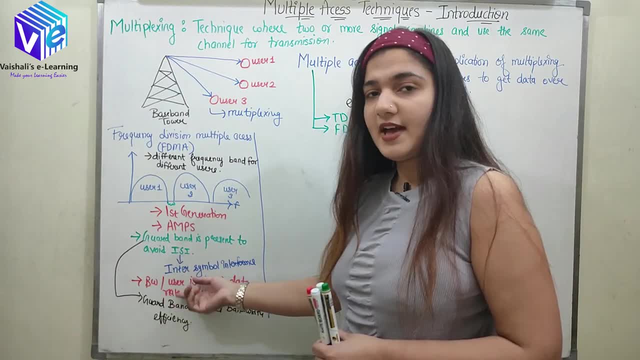 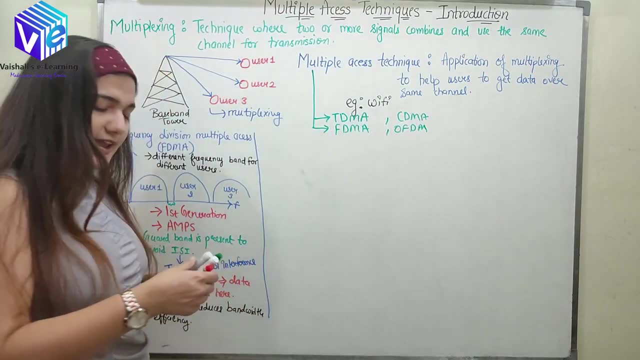 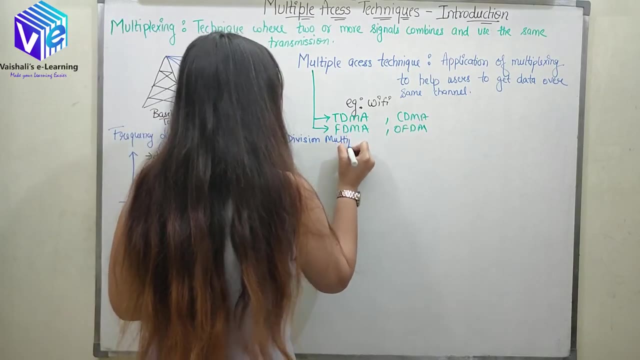 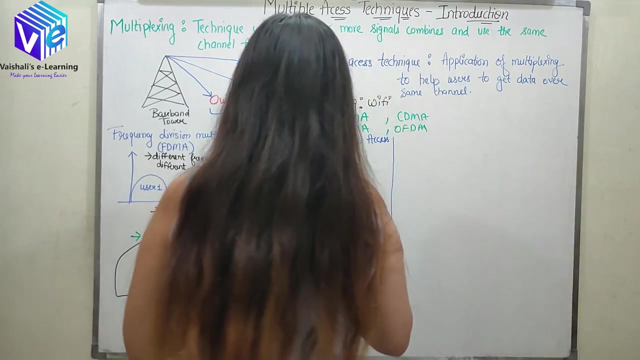 So because of this guard band, it is becoming very costly, So I have to remove this guard band also. So now the next technique which came in the second generation data transfer was time division, multiple access, or it is called TDMA. So now here, what? here we had different frequency bands. 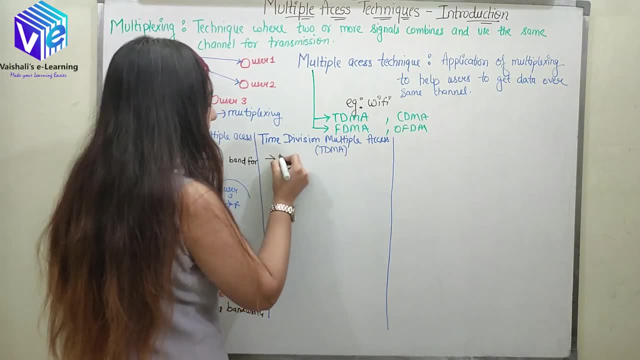 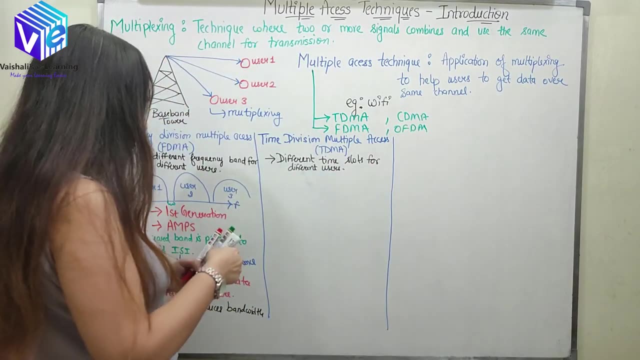 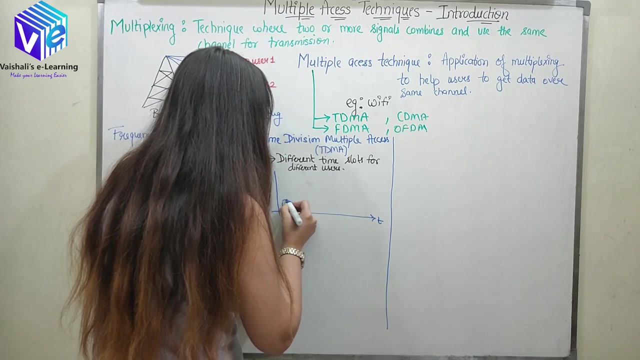 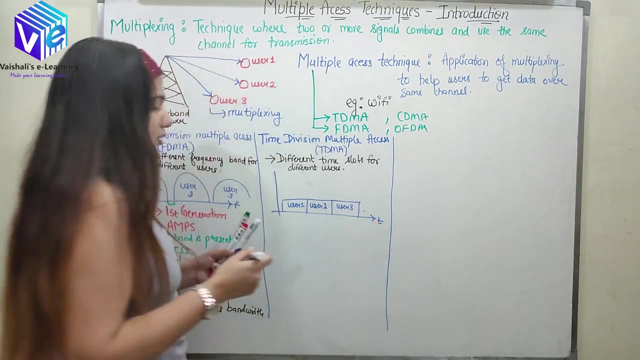 For different users. So here obviously we will have different time slots for different users. So now, if I have to plot it on the time axis, So now if this is my time axis, So this would be my user 1, this would be my user 2, user 3, and so on. 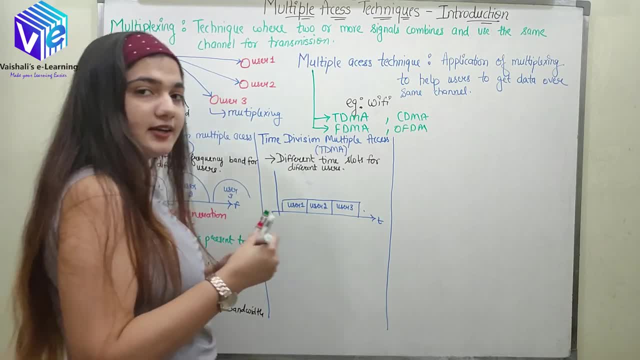 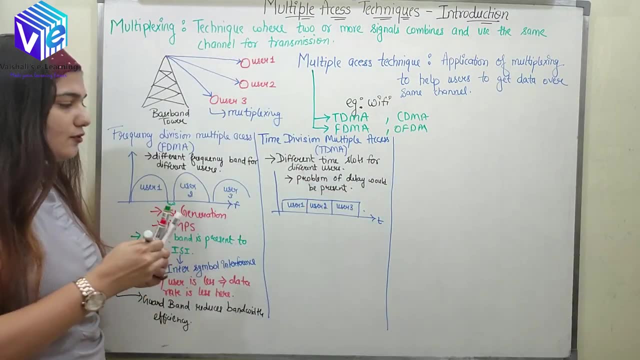 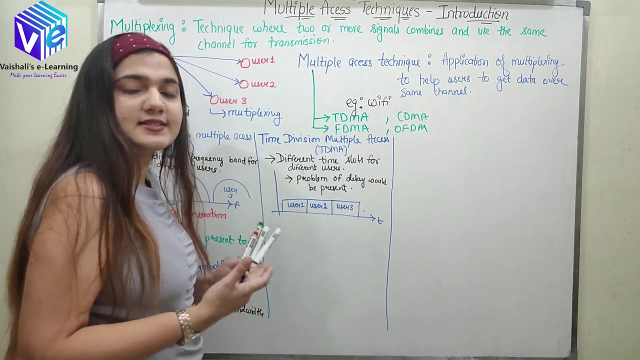 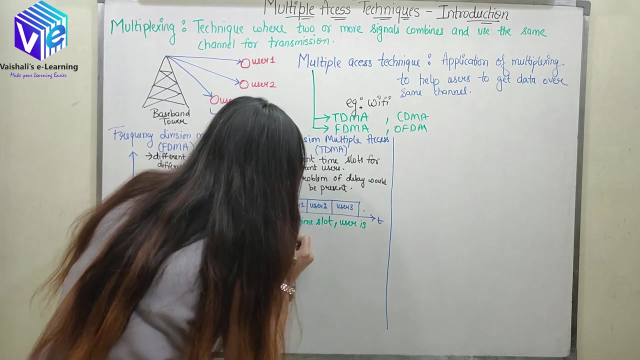 So now you can see different people are using different time slots. So here is the problem of delay. So the user 1 is using the first time slot and it is using the full frequency band in the first time slot. So in a particular time slot, 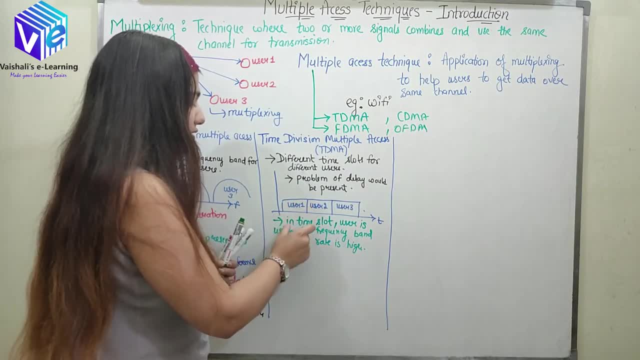 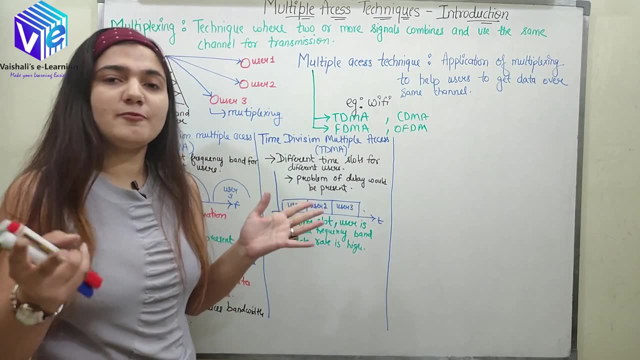 So because in the particular time slot the user is using the full frequency band. So If I have the particular time slot in my time slot I'll be using the full full frequency band. So in that time slot I'll be getting more data rate. 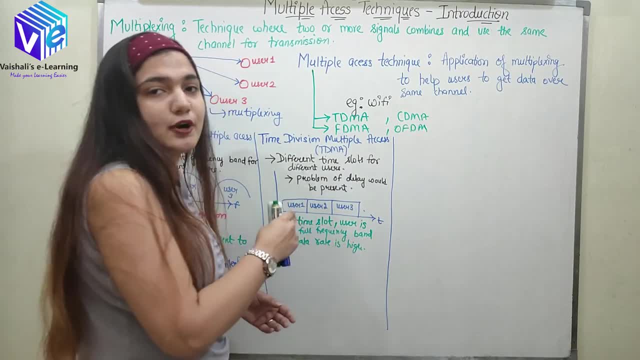 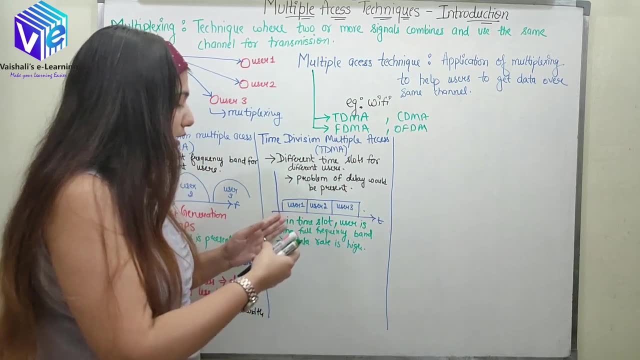 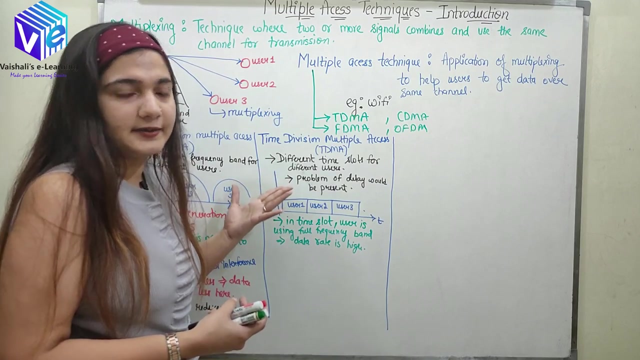 So the data rate is high in the particular time slot only, But if I have to again use it, I have to wait for my slot to come again. So now I hope you understand what is time division, multiple access, and I hope you can see here there is no guard band. 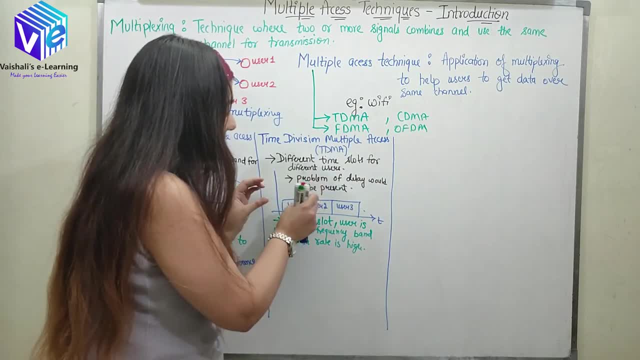 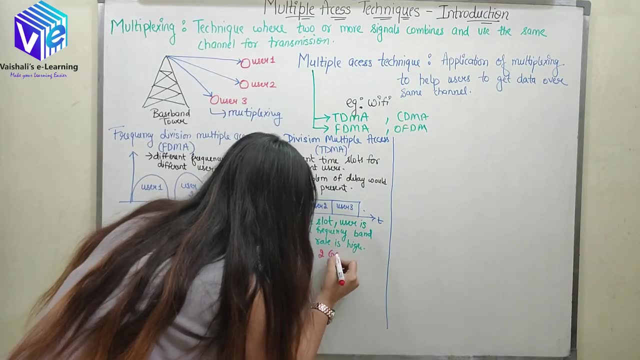 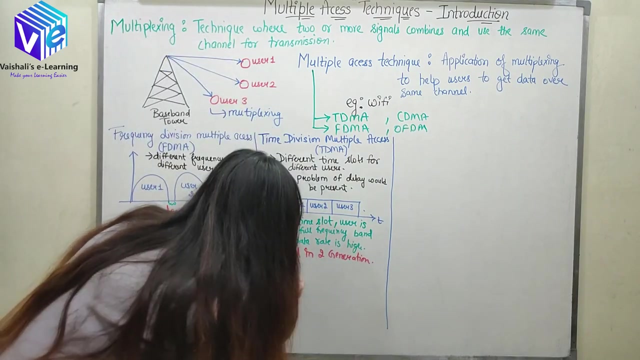 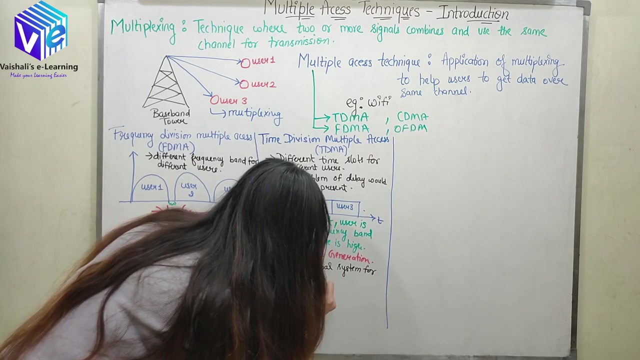 So I don't require different Okay, Guard bands between different users. I hope you understand this. So now it is used in. It is used in second generation data transfer. So let me give you some examples. So the first example is GSM, global system for mobile communication. 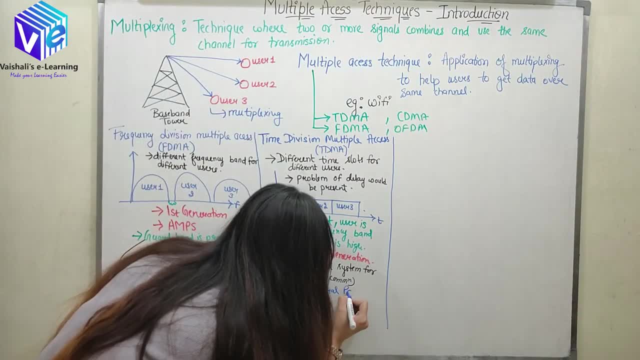 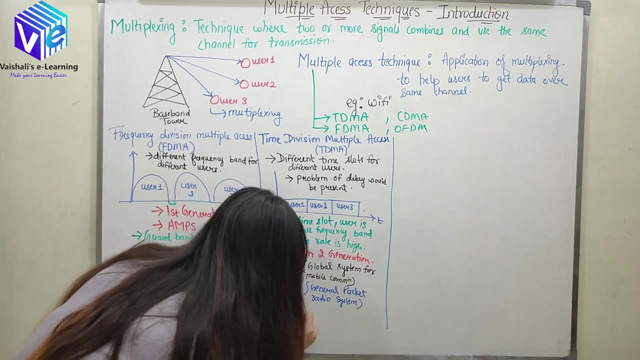 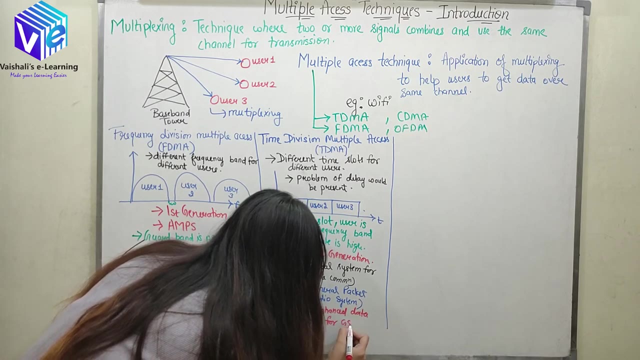 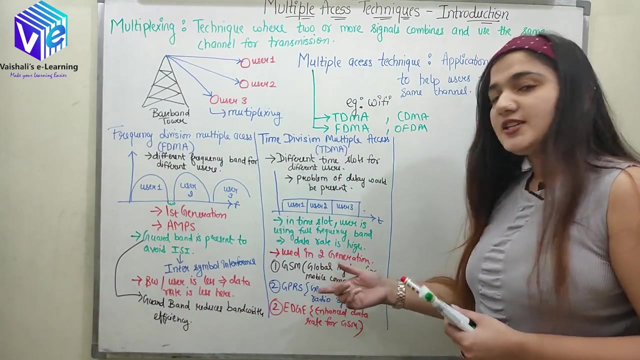 Second is GPRS General packet Radio system, And third is edge Enhanced data rate for GSM. So now, I hope you all have heard about these terms, So these are used in 2G communication. So now coming to the next technique. 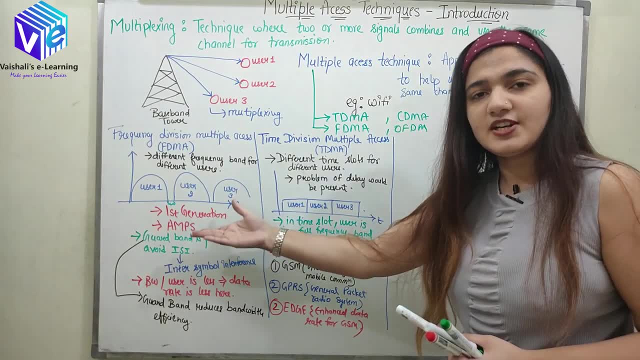 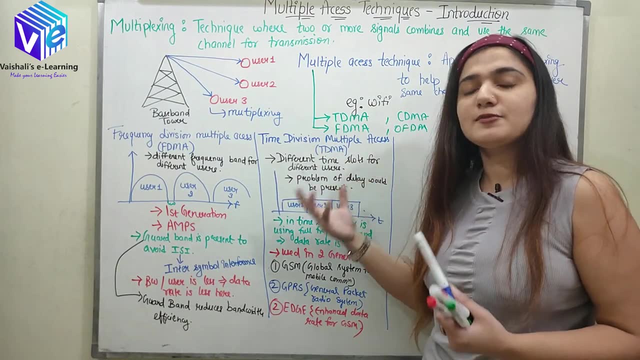 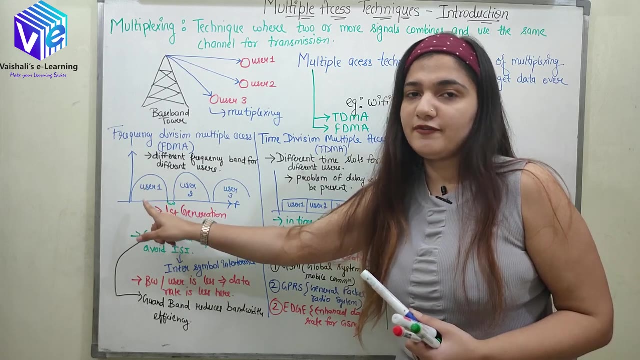 So these had some drawback. The first First generation Technique Drawback Which was overcome by the second generation. So in the second generation we were using the full spectrum, the full bandwidth spectrum for a particular user. here The spectrum was limited, because of which the data rate was less here. 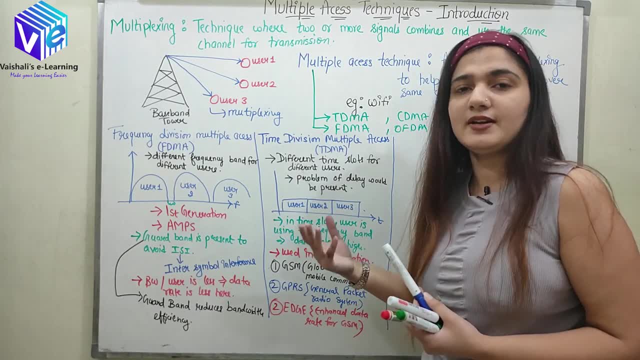 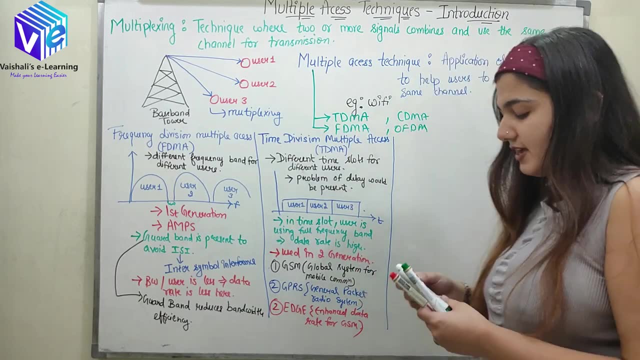 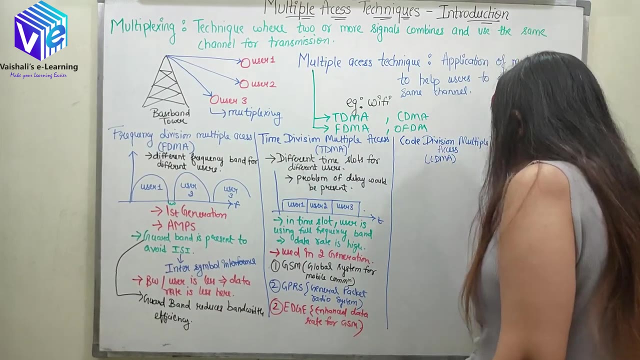 The spectrum was full, but the time slots were different, because of which delay was present. So now I have the third multiple access technique, which is called the CDMA, which is code division multiple access. It's basically looking through the exerge, and so I have already talked to you about 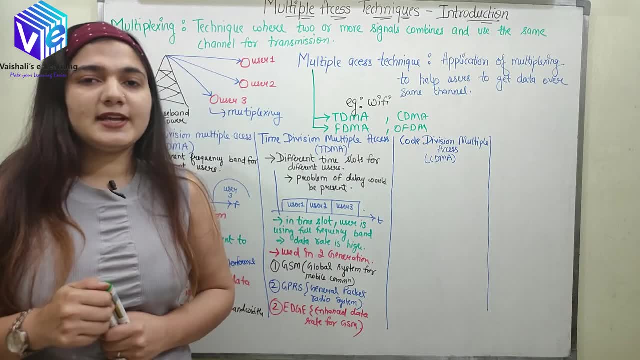 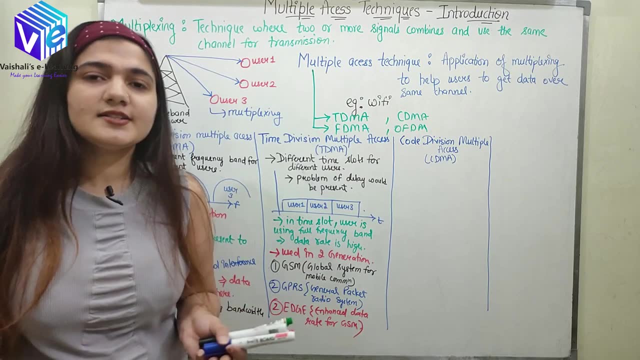 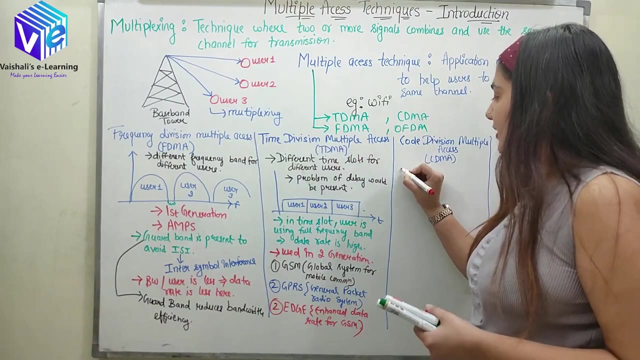 the spread spectrum technique. So in the spread spectrum technique I told you, I have a pseudo-random code which is multiplied with the message signal to enhance its bandwidth. Same thing is happening here. Here I have a pseudo-random code which has multiplied with the message signal. 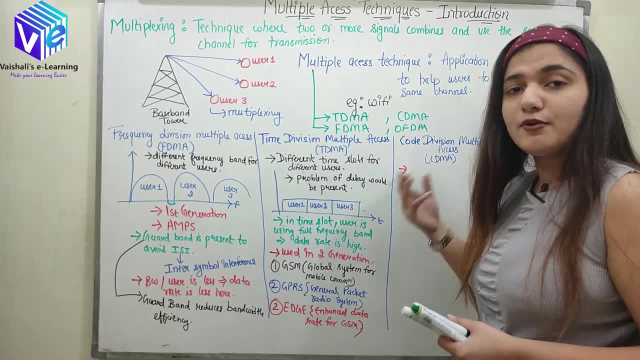 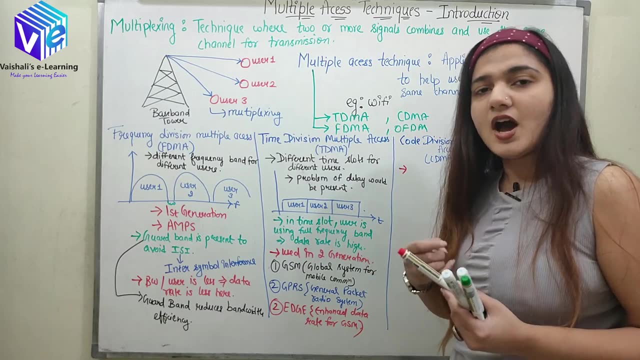 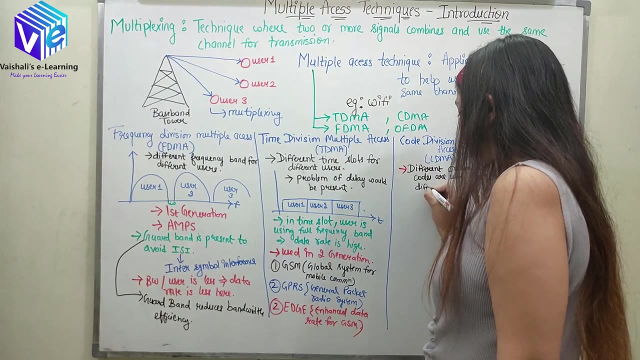 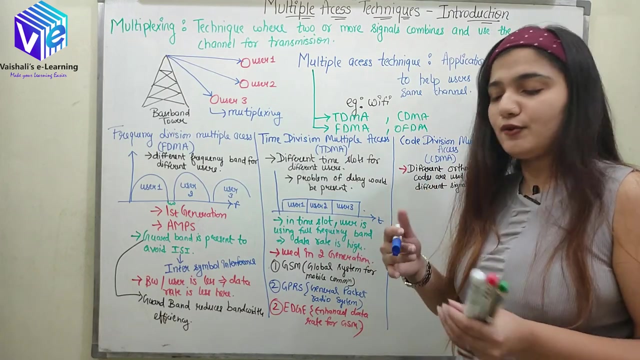 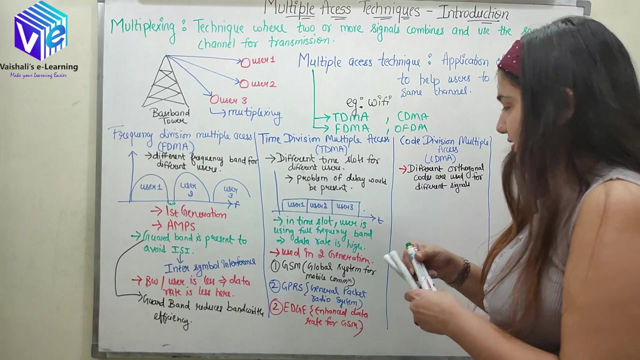 So now in this, different orthogonal codes are taken For different signals and different signals superimposed on different orthogonal codes are sent on the same channel. So the orthogonal codes are multiplied with the signal and it is sent over the channel. So now, when this thing happens, there would be the problem of inter-symbol interference. 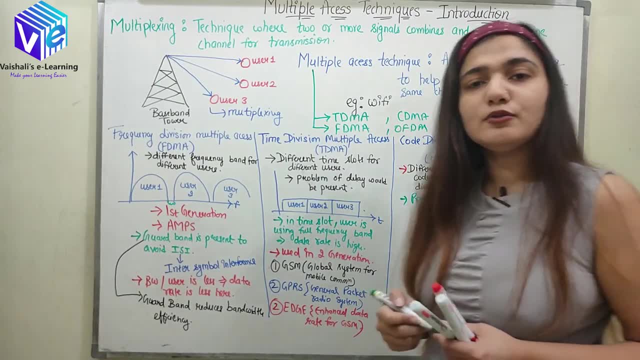 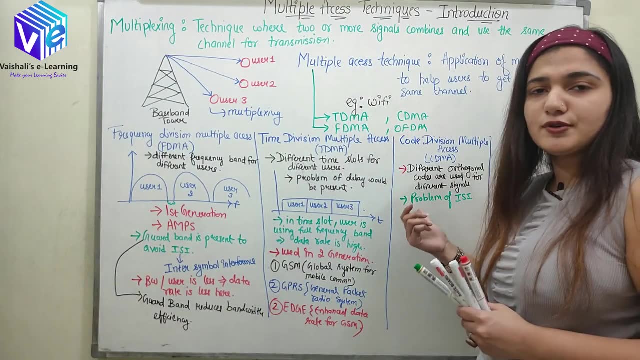 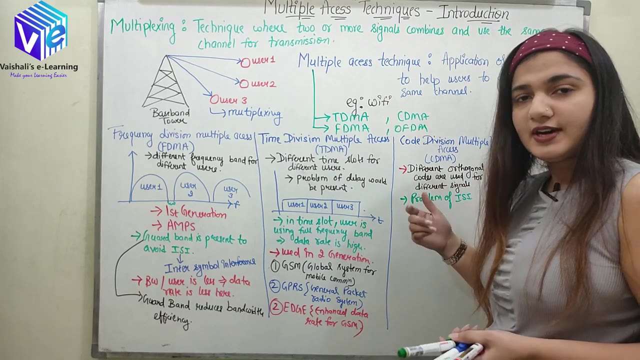 When I will talk about CDMA in detail, I will tell you how this inter-symbol interference is happening. So as of now, you should know, in CDMA there is the problem of inter-symbol interference. So now here, I am using different codes per user, So if I have multiple users, 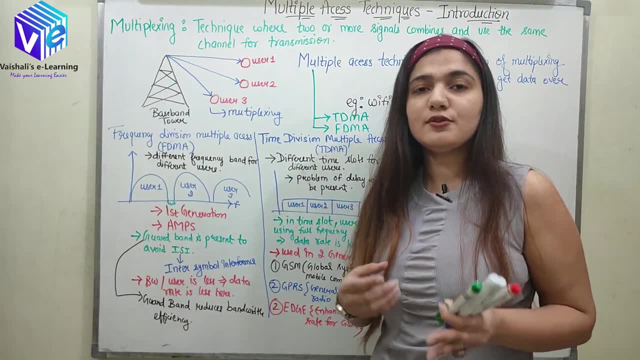 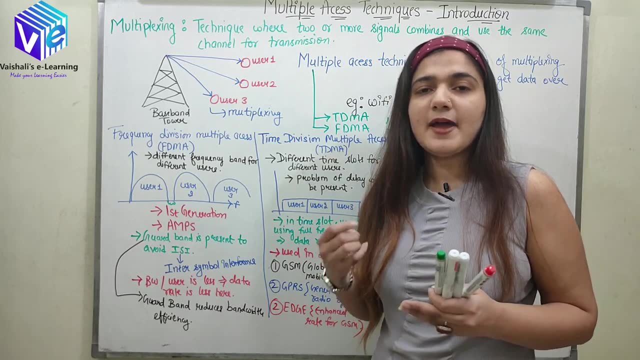 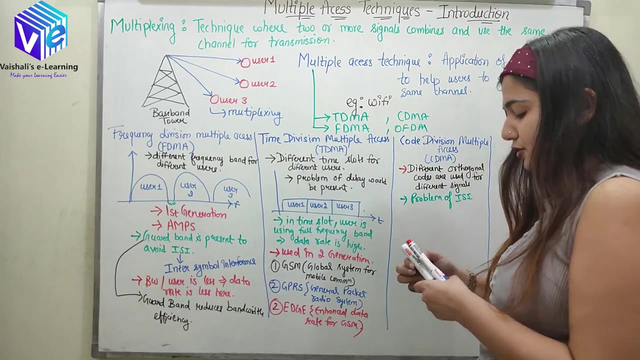 I will be having multiple codes and at the receiver also these codes are multiplied. Like the same way I did it in CDMA In spread spectrum technique. in the spread spectrum I multiplied the pseudo random code at the receiver also. So here the same code is multiplied at the receiver also. 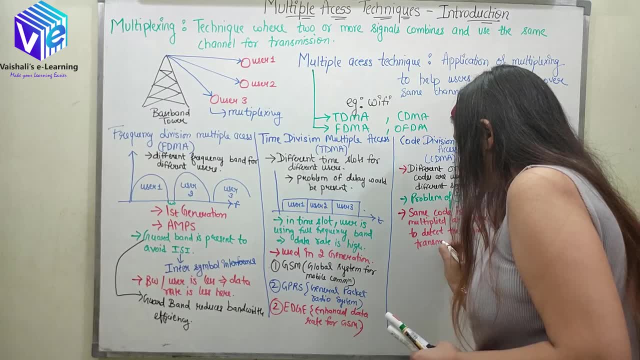 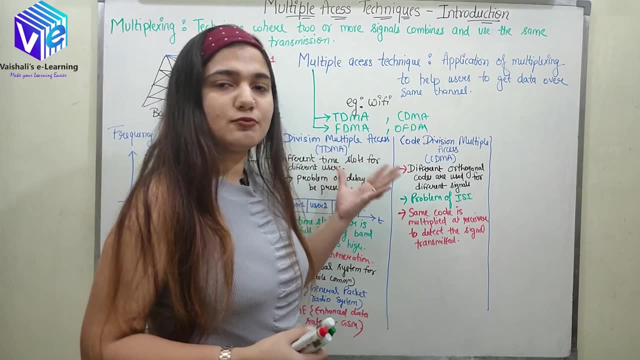 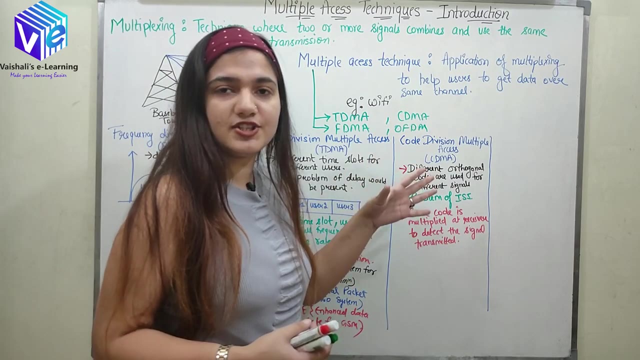 So I hope now you must be imagining what would be happening in CDMA. So in the CDMA the pseudo random codes are there for different signals, Some orthogonal codes are there which are multiplied to the signal and sent to the channel. In the channel they won't get. 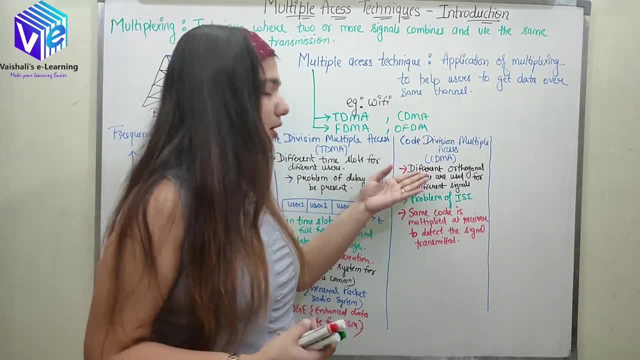 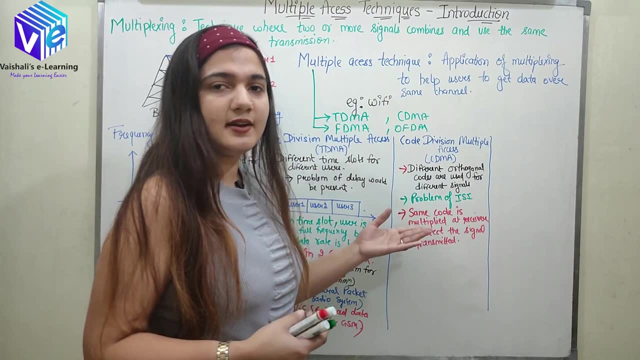 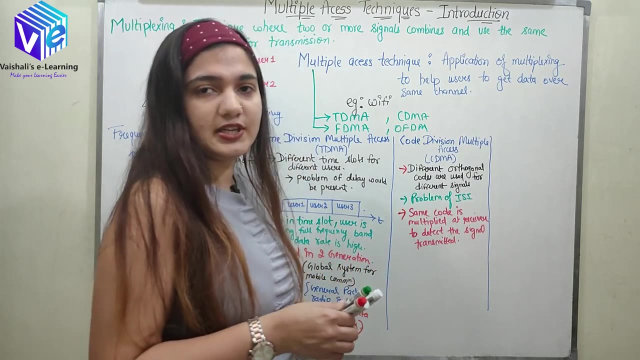 mixed up because these codes are orthogonal in nature. So I will explain you and I will talk about CDMA. So now at the receiver also, these codes are multiplied again and the codes which we sent, or the signals which we sent, are detected back. So it is used in 3G communication. 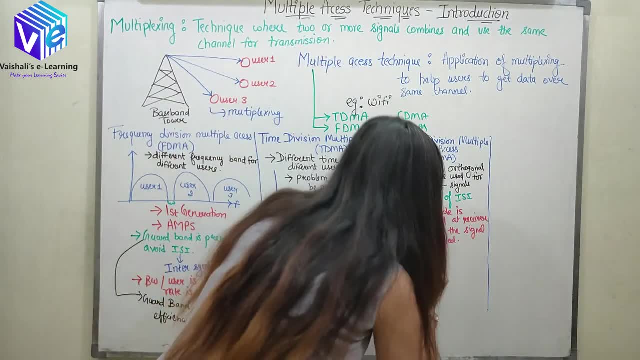 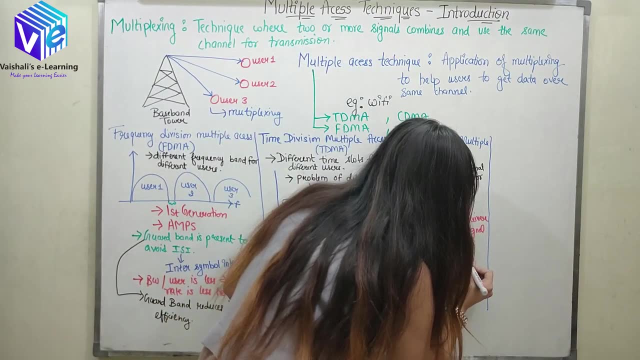 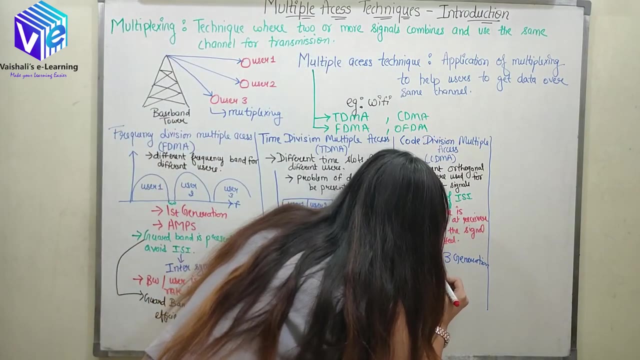 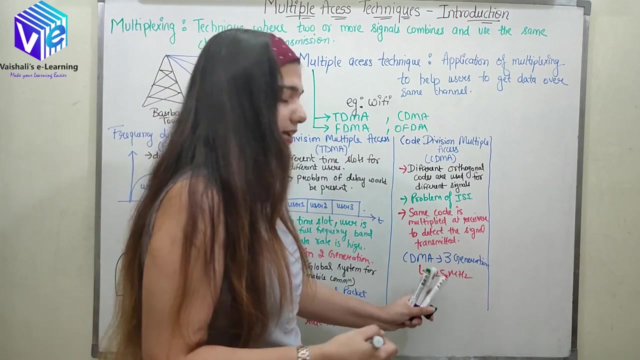 I hope you have heard about 3G communication. This is used in 3G or 3rd generation. So it is using the frequency band of 1.25 megahertz. So this frequency band is again less. So to improve upon the frequency band, WCDMA technique. 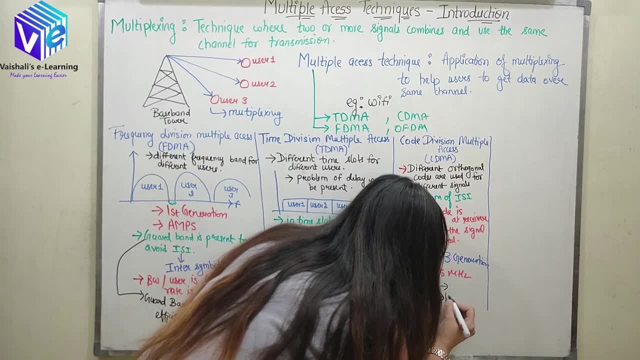 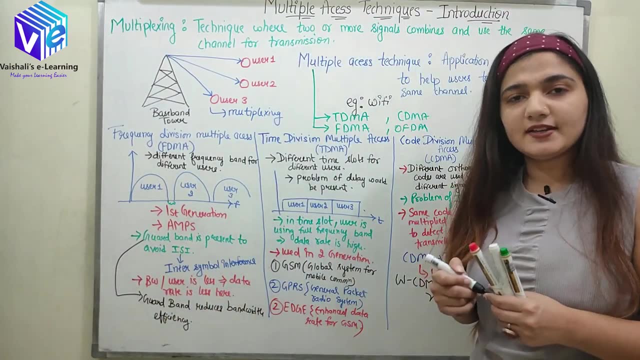 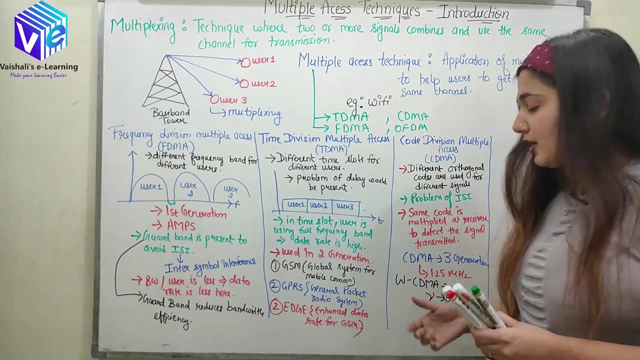 was used. So it has the frequency band 5 megahertz. WCDMA technique has the better frequency band, So if it has large frequency band then obviously the data rate here would be better. So WCDMA technique had better data rates. 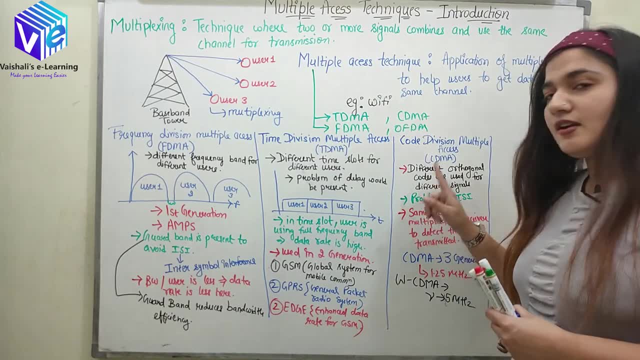 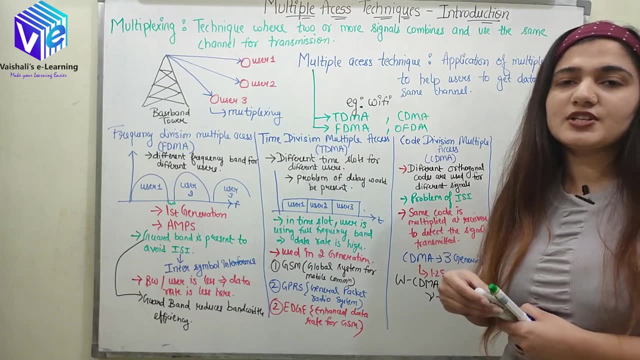 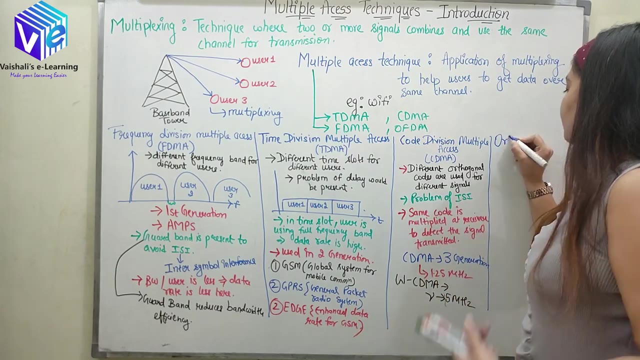 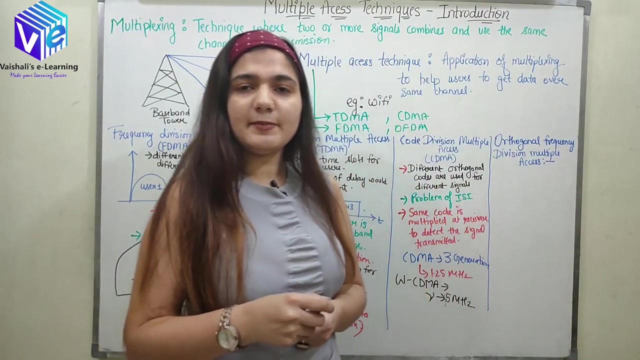 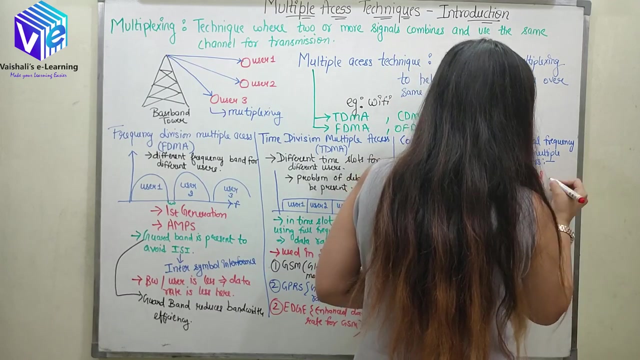 than CDMA technique. So now if this signal also had the problem of inter symbol interference? So another coding technique was introduced, which is orthogonal frequency division- multiple axis. So orthogonal frequency division- multiple axis is a technique where orthogonal subcarriers are used. 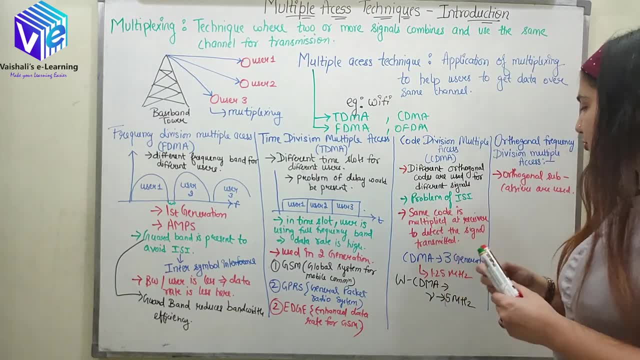 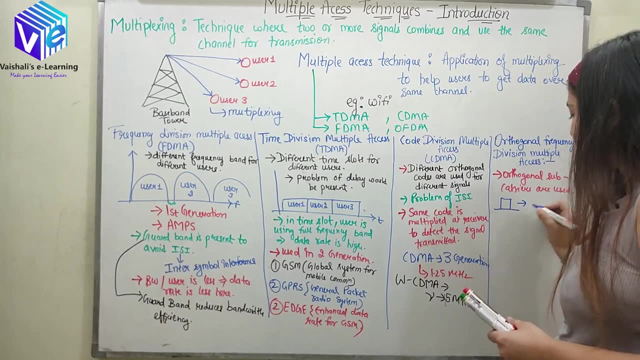 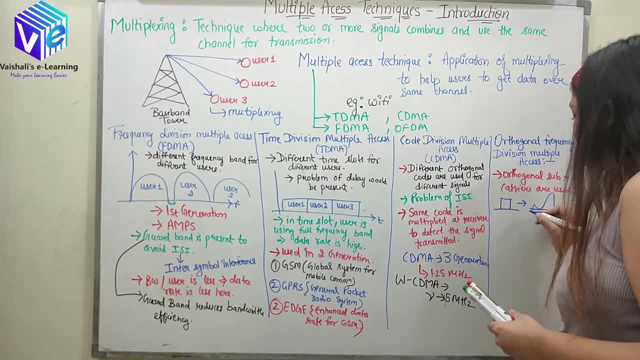 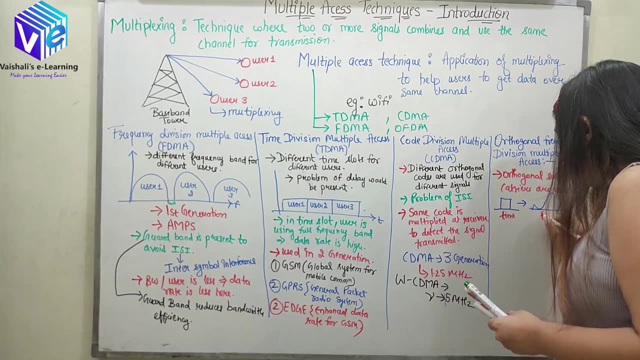 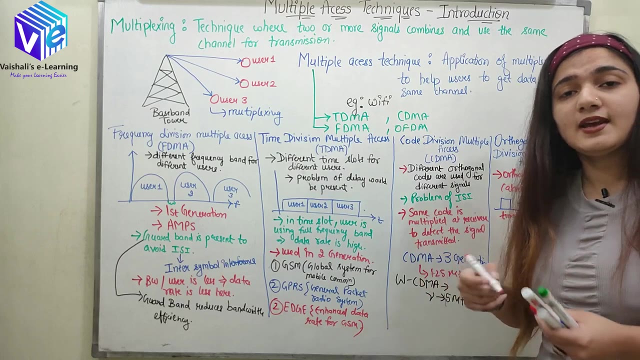 Then its frequency spectrum would be in the sink function. So now this is in time domain and this would be in frequency domain. So now if I choose different subcarriers whose frequency domain are orthogonal to each other? So now if I talk about different subcarriers? 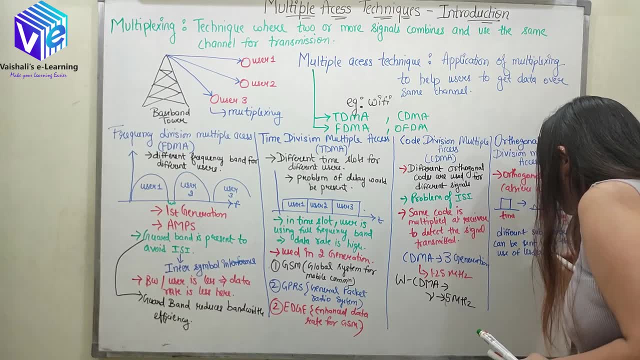 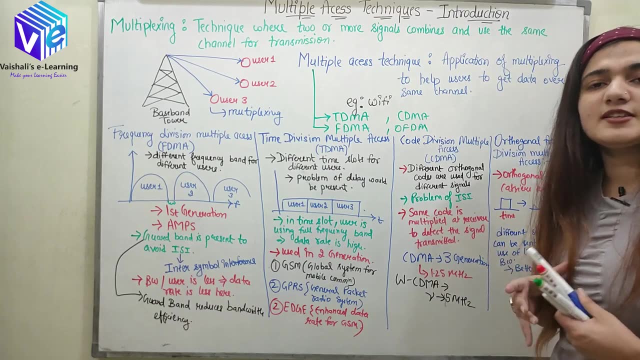 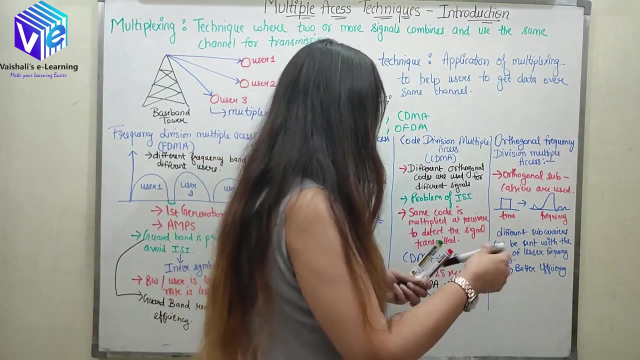 So if I talk about different subcarriers, So different subcarriers can be sent with the use of lesser frequency bandwidth. When I will talk about OFDM, I will tell you how the frequency bandwidth is reduced. Here we don't require actually guard band. 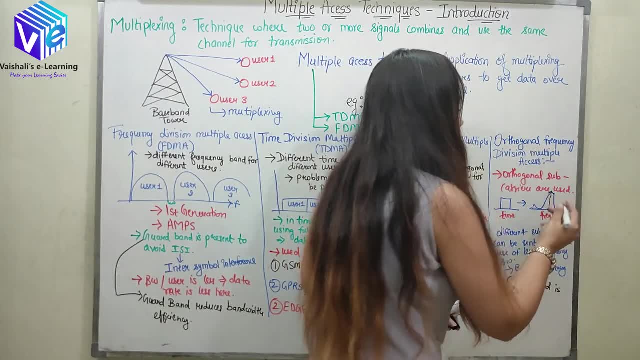 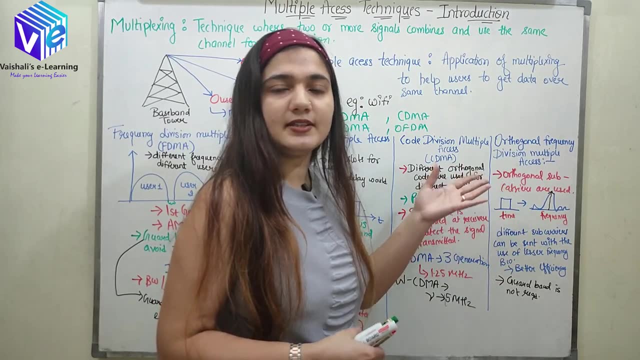 So what can happen? if this is my subcarrier 1, the subcarrier 1 can be superimposed on the subcarrier 2, similarly, which can be superimposed on the subcarrier 3, and that is how I can superimpose them and save my frequency band and transmit to the channel. 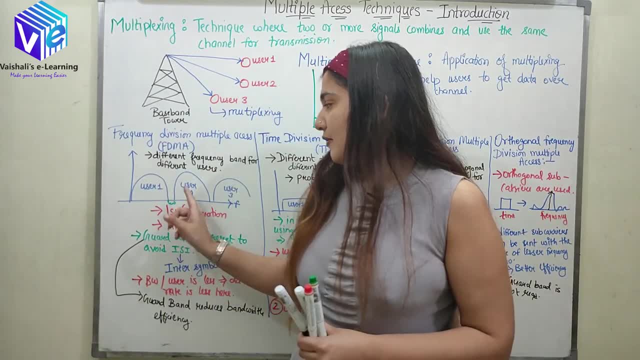 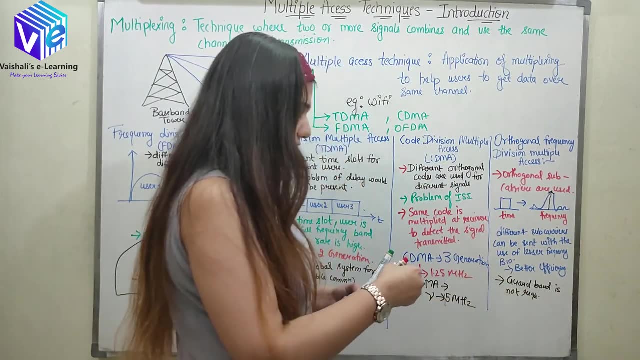 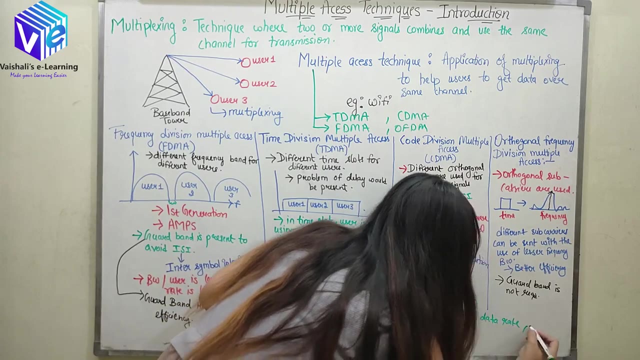 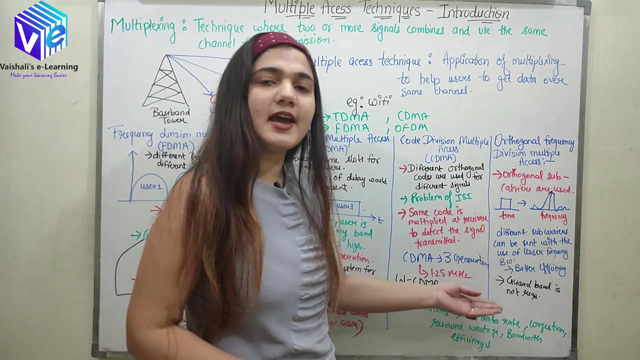 So these will not get mixed up like in FDMA. what we had, we had a guard band. here the guard band is not required. So now here in WCDMA we had some limitations also, So the limitations are. so the limitations are less data rate. 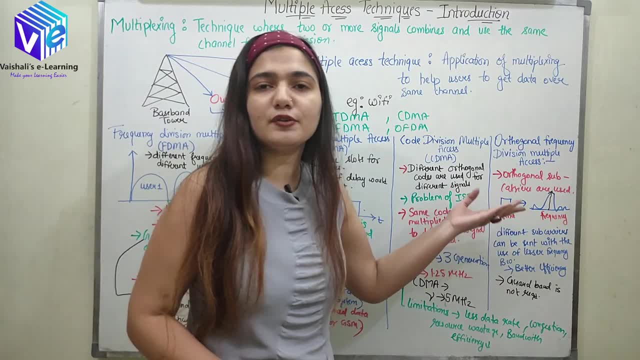 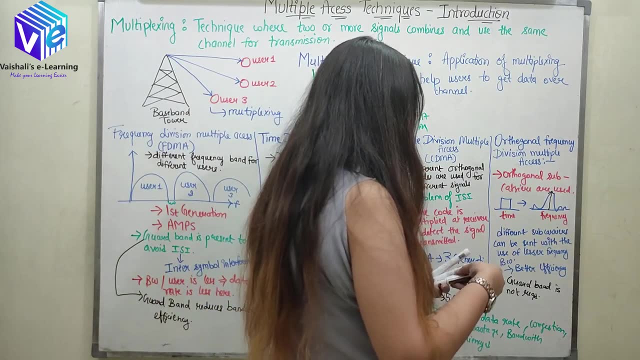 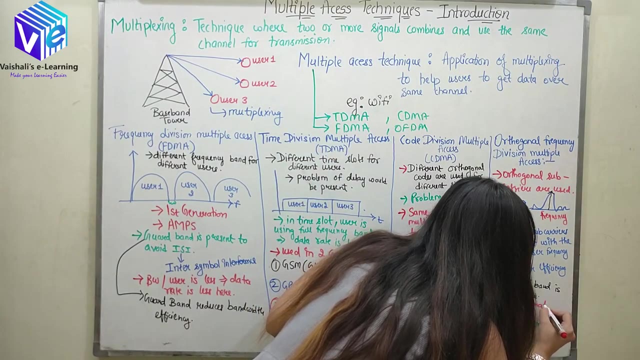 It has comparatively less data rate when I compare to Orthogonal Frequency Division Multiple Axis. This is my 4G. Orthogonal Frequency Division Multiple Axis is the 4G communication. So here 4th generation data transfer would be there, or LTE data transfer would be used. 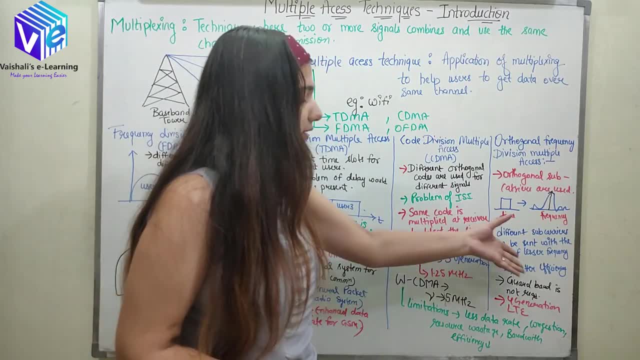 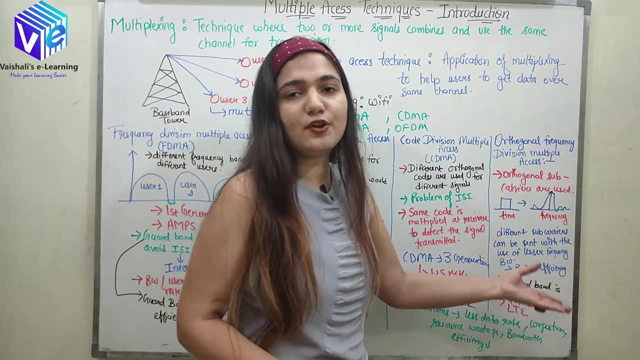 which is called long term evolution. So now here the data rate would obviously be better. So Here we have less data rate and here we have congestion of users at the peak time. At the peak time, a lot of users would try to access the data, so there would be congestion.